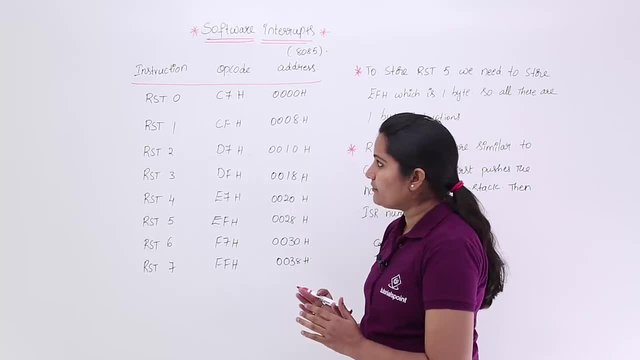 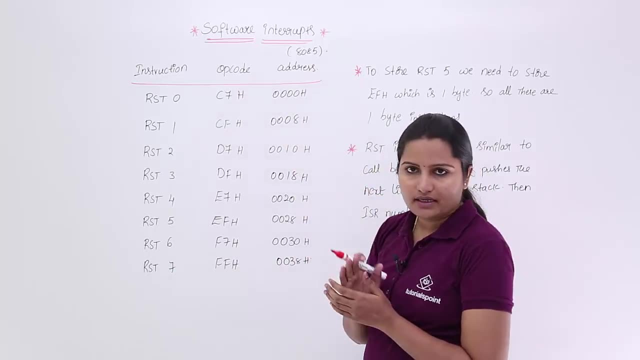 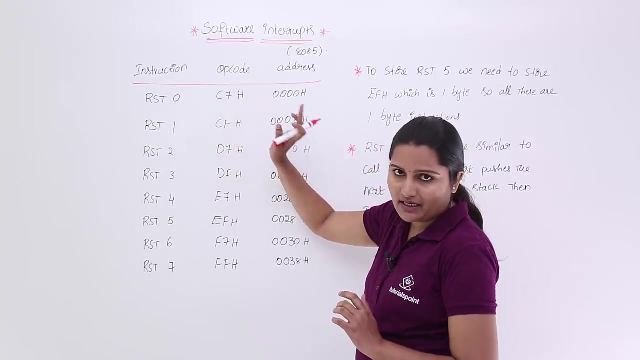 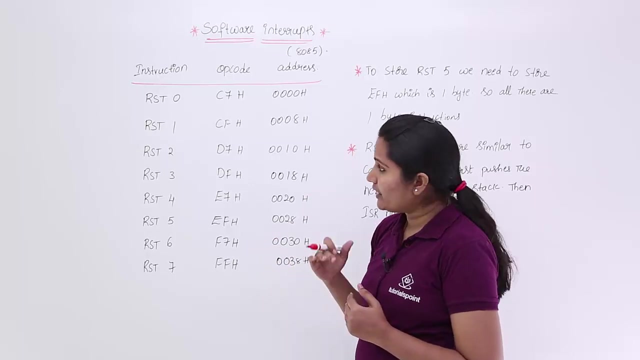 These are the software interrupts we are having in 8085. RST0 to RST7 are the software interrupts, and the opcode and address are given as follows. So here the opcode for RST0 starts from C7H, and by adding A to C7H we are getting opcode for RST1. 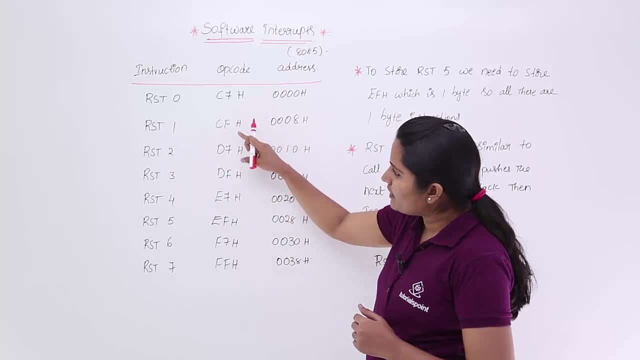 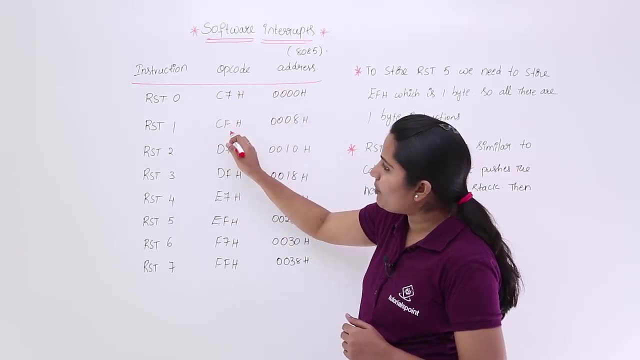 So you can observe, for in between each and every one of these, everything we are having 8, 8, 8 difference. that means, by adding 8 to C7H, you are getting the opcode for RST1. by adding 8 here, you are going to get D7 here. by adding 8, here you are getting. 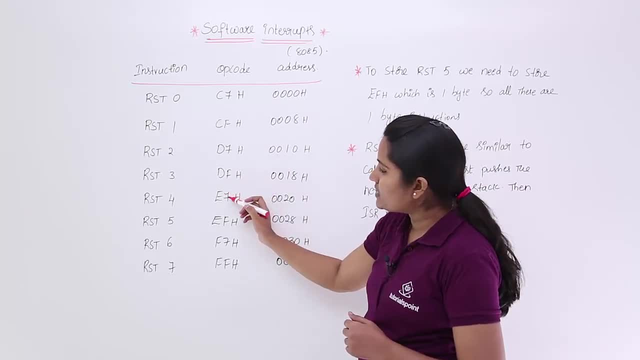 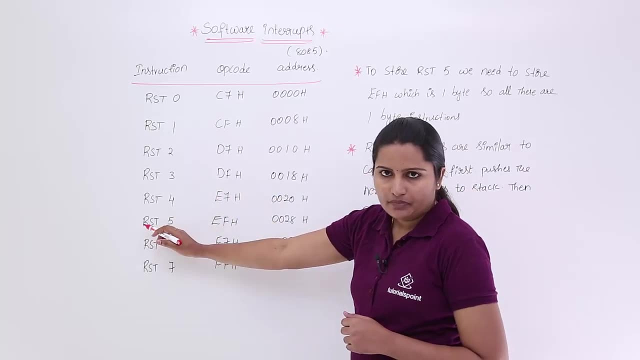 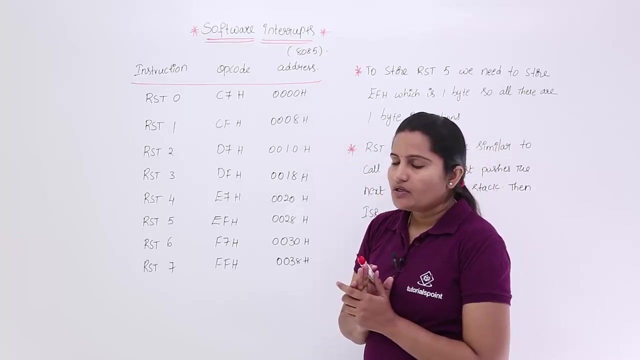 DF here and like that, by adding 8 here you are getting E7H. by adding 8 to E7H you are getting EFH, which is the opcode for RST5.. Now coming to the address, so you can see you are having instruction, opcode and address. how we can get that address means, for example, if you are having 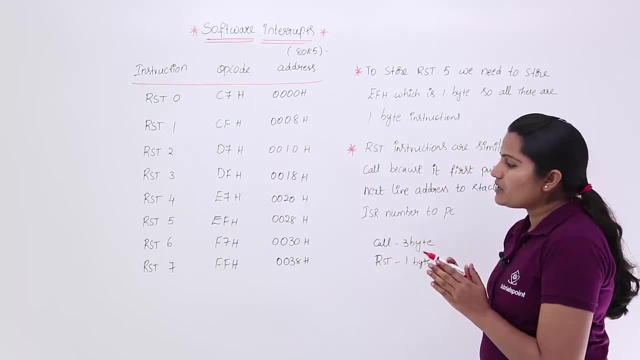 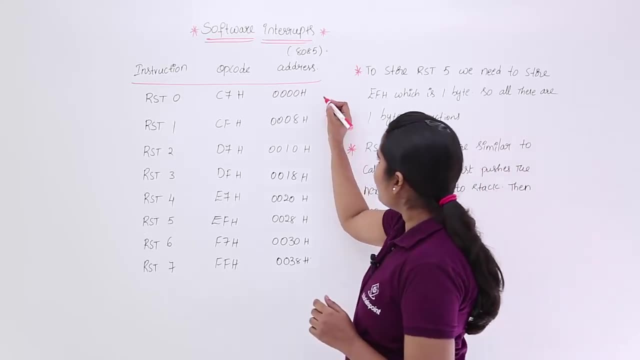 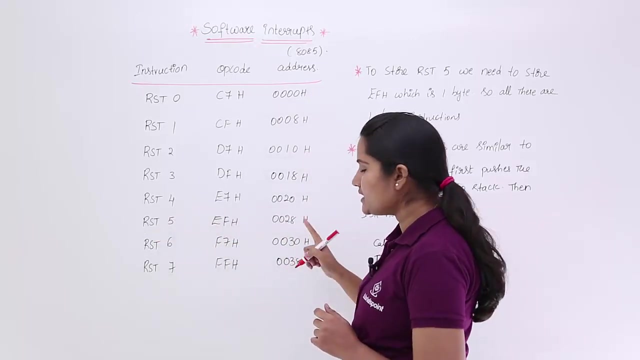 RST5, then the address of RST5 can be found by multiplying with 8. that means 8. For example, if you want to find out the address related to RST 5, if you do not know this, then you can write like this: that means 5 into 8. you can write like this: and this is: 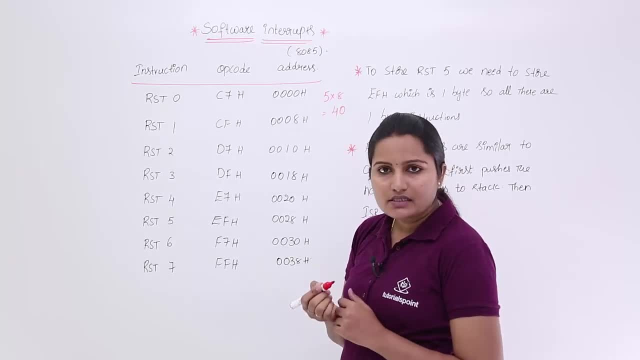 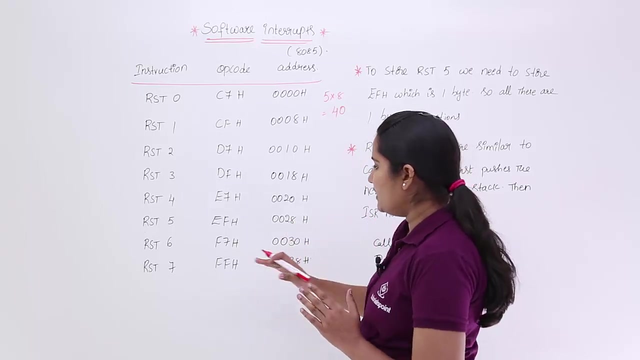 equivalent to 4, 0, but this 4, 0 in hexadecimal is equivalent to 2, 8.. So the address is equivalent to 0, 0, 2, 8 H. So similarly so for RST 6, if you want the. 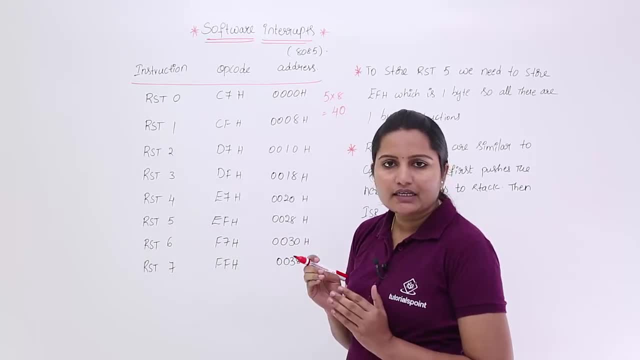 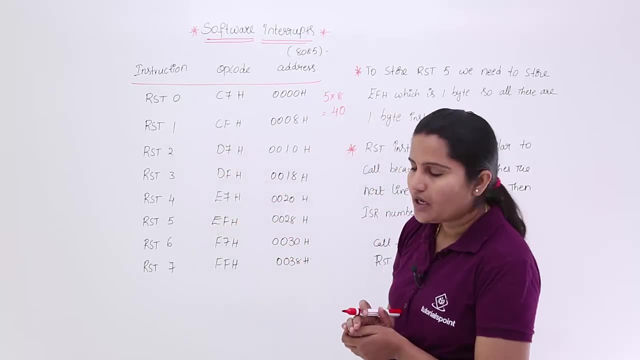 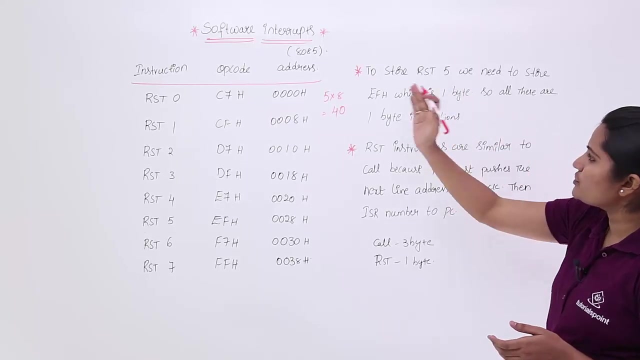 address. just multiply 6 into 8 and the result you can convert into hexadecimal. you can get the address of each and every instruction. So now coming to the important points related to software interrupts. to store RST 5, we need to store the address. 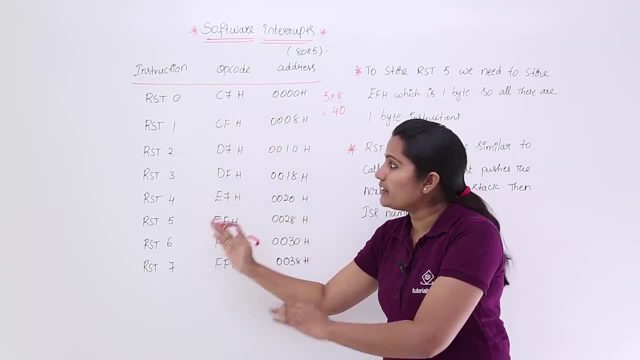 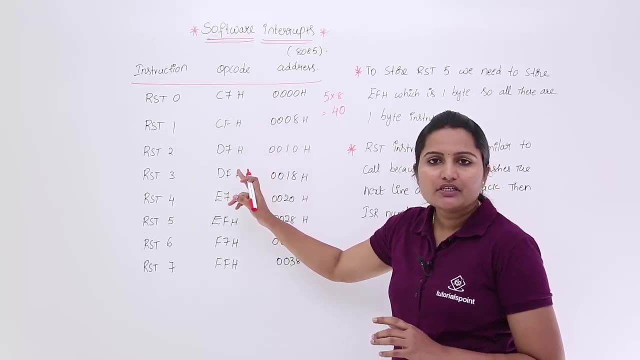 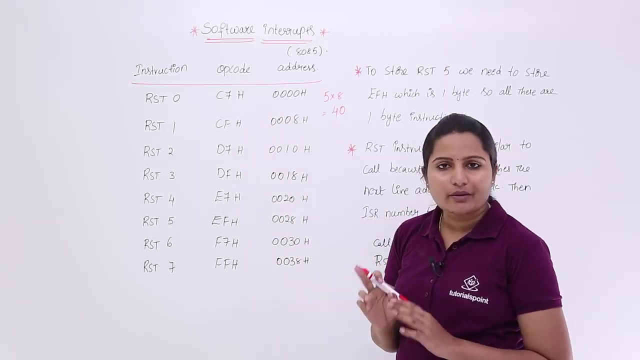 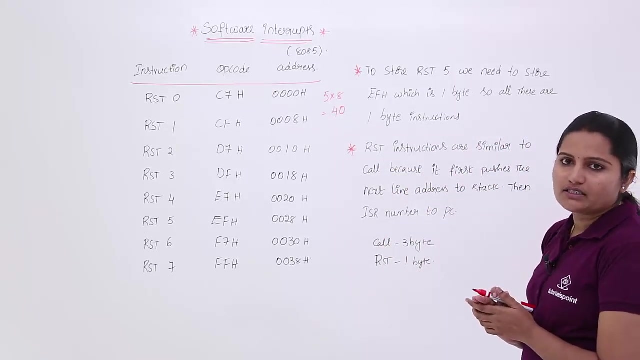 So we need to store the opcode. first, to store any interrupt, we need to store the corresponding opcode. that means each opcode. if you observe that will source 1 byte. So all these instructions, software interrupts, all these interrupts are 1 byte interrupts. and now coming to RST instructions, which are very similar to call instructions. that means: 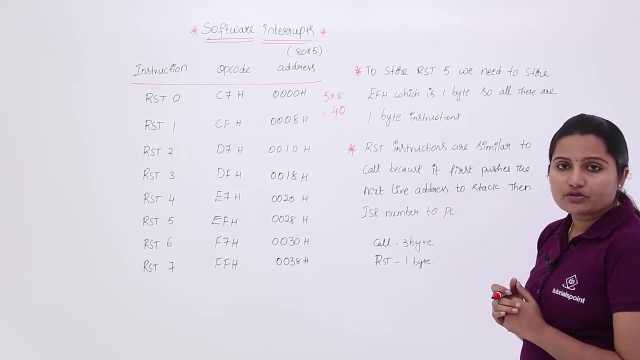 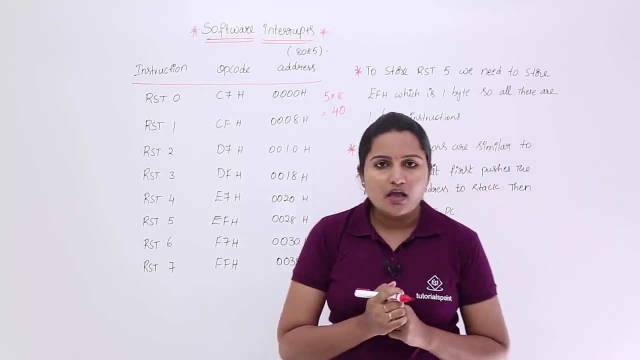 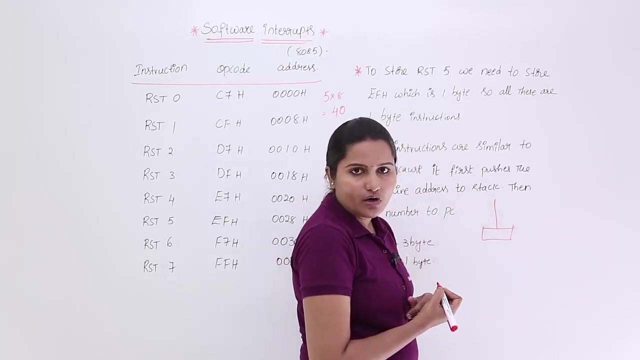 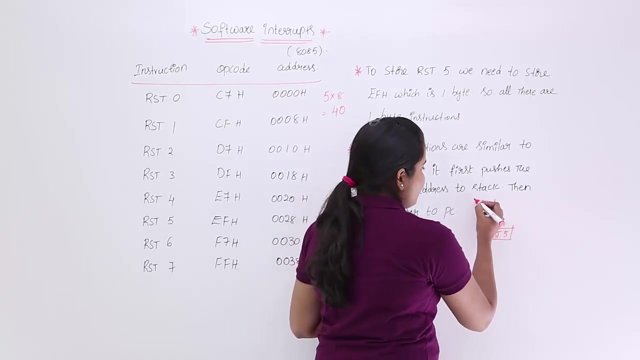 before getting into interrupt service routine, These instructions are going pushing their next address to stack. For example, if you are in a program you got some interrupt, So here you got interrupt, So RST 5 you got here, and what you are doing here means, for example, you started your program. 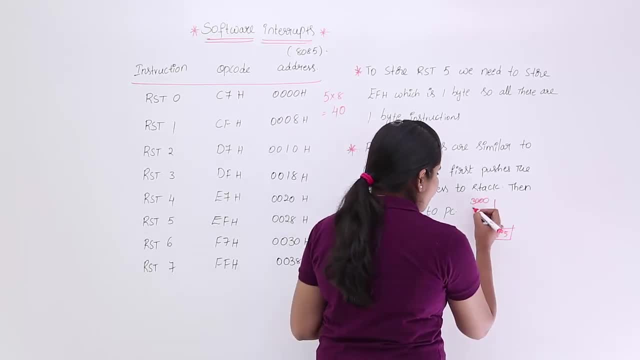 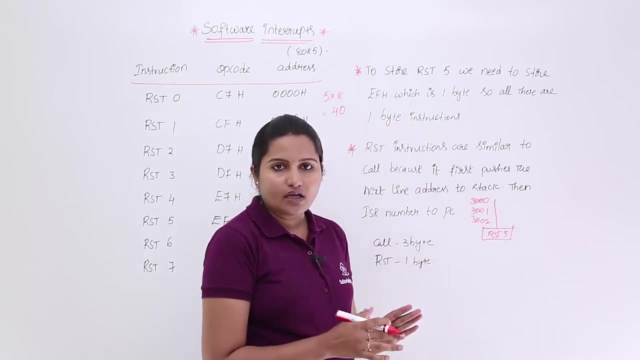 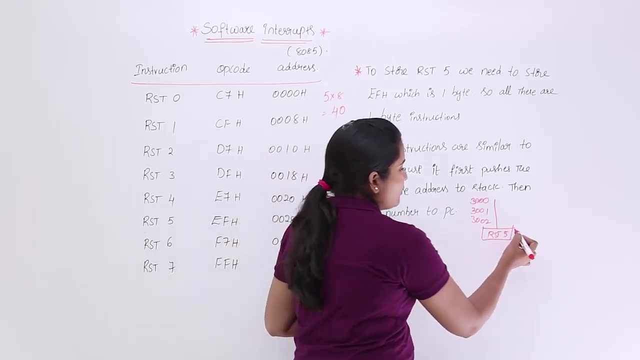 at 3000 location and you executed 3001, 3002 up to 3000.. to you executed the program after 3002 at 3002, you got, or you encountered, an interrupt. then, before getting into this interrupt service routine ISR path, it is filling the stack with. 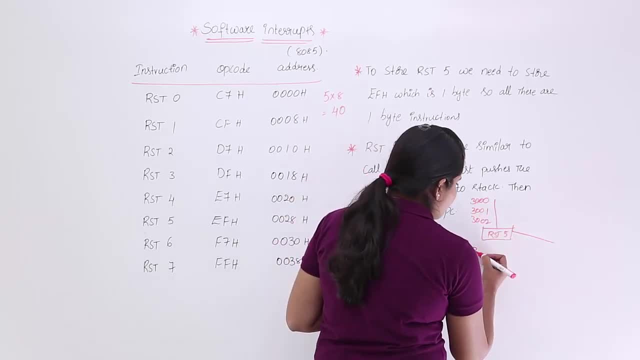 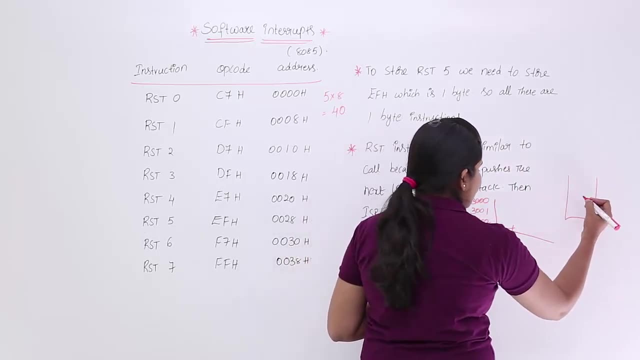 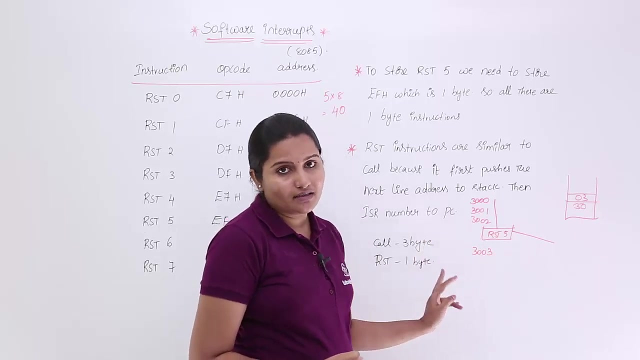 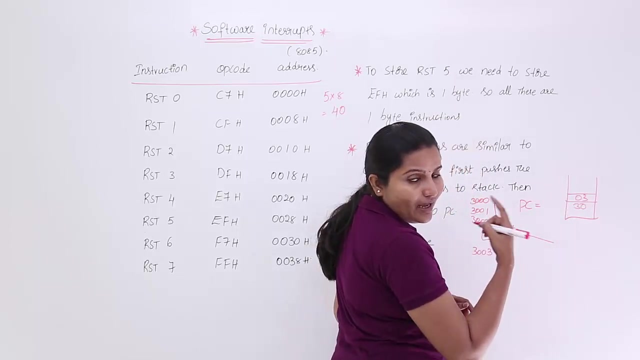 its next address. that means its next address is 3003. now it is pushing the contents of next address into the stack. that means so now the stack register is going to fill with this data. that means next address data, and so it will takes the program counter as ISR. 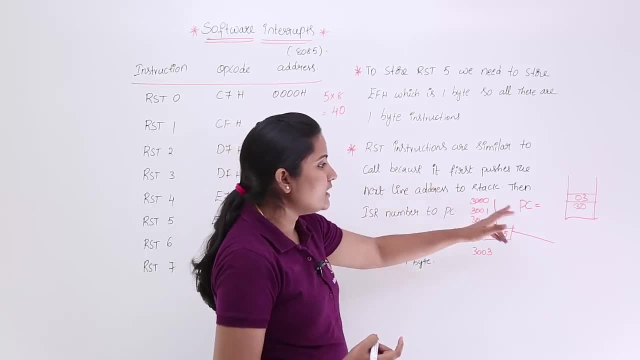 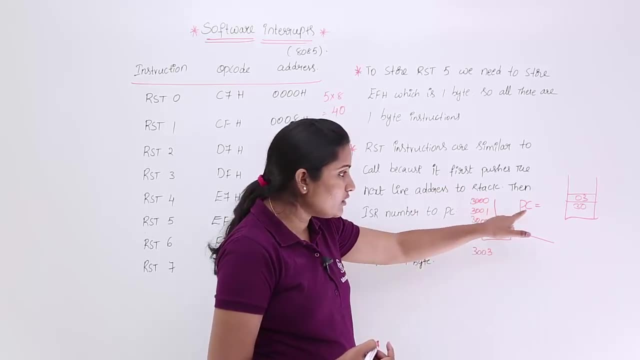 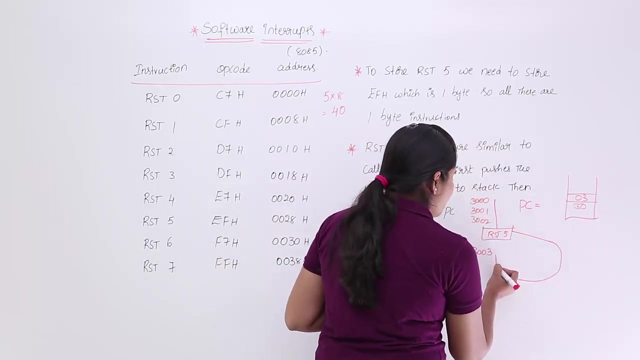 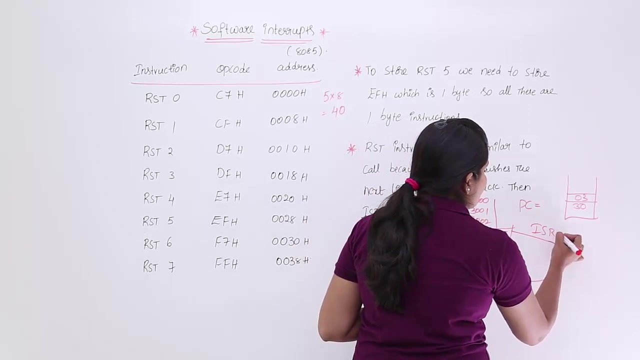 that means so whatever ISR number is there that will take here that means to which that interrupt is pointed to that location your program counter is loaded. So after completion of this task again your program control will come to this location. so this is called as interrupt service routine. so now you can observe if any interrupt came. 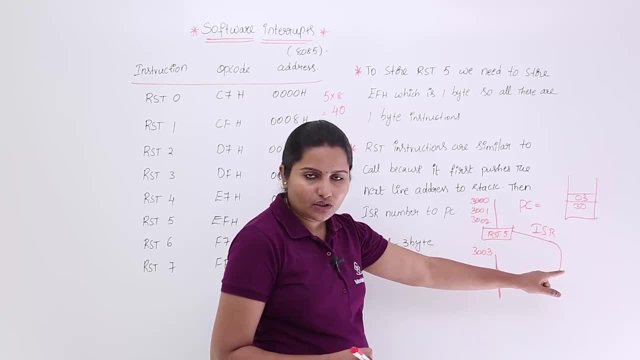 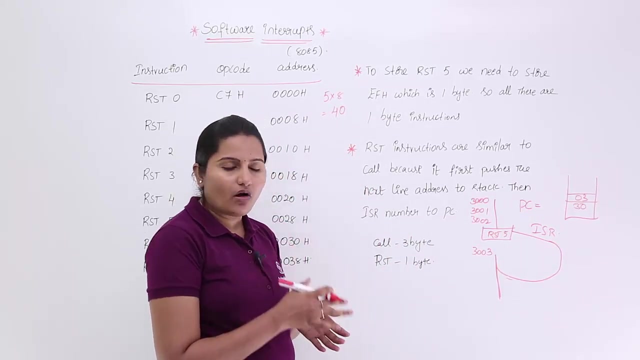 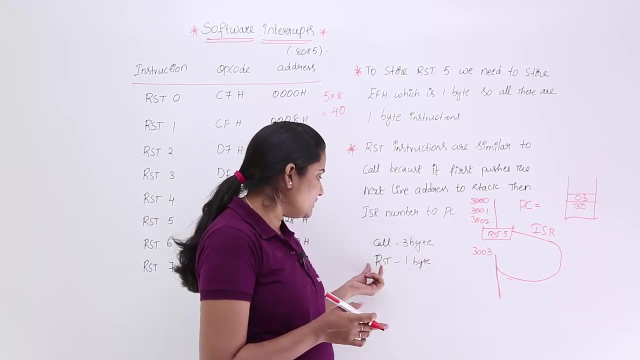 software. interrupt came before getting into the service routine. it is pushing the data of or address of next instruction or next location to stack. So this is somewhat simple. Similar to call instruction, only so here the only difference between call and RST instructions or interrupt is so call instruction is of 3 bytes and these interrupts are 1 byte, so